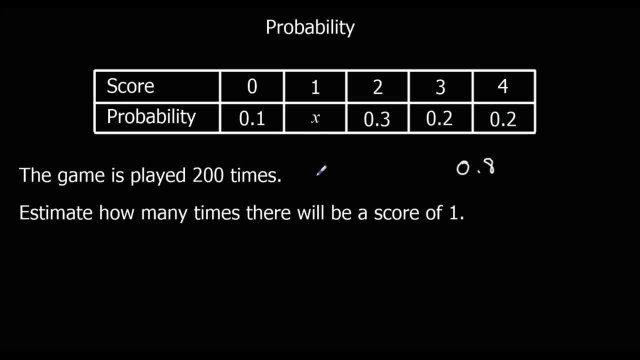 So so far we've got 0.8, and they need to add up to a whole. So that means the missing probability here has got to be 0.2, because 1 minus 0.8 is 0.2.. 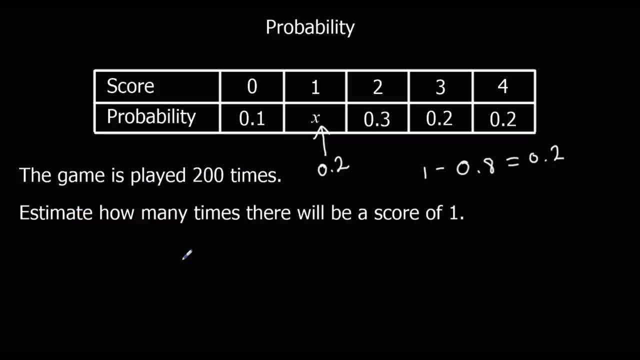 Now it says the game is played 200 times. Estimate how many times there will be a score. So it's this decimal, this chance, times 200.. So it's 0.2 times 200.. We want this fraction. If it was a fraction, it would be one-fifth, one-fifth of 200.. 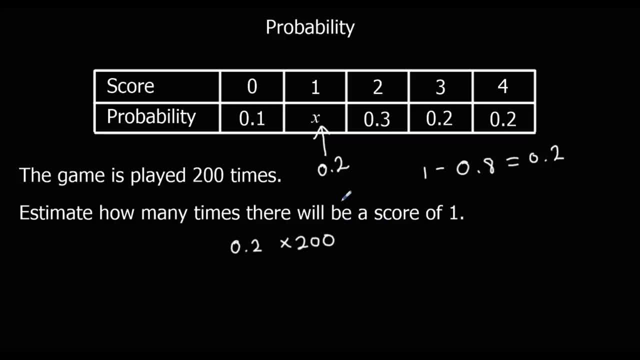 If it was a percentage: 20%, 20% of 200. So it's just 0.2 times 200.. So 2 times 200, that's 400.. But because it's 0.2, we take off a zero. 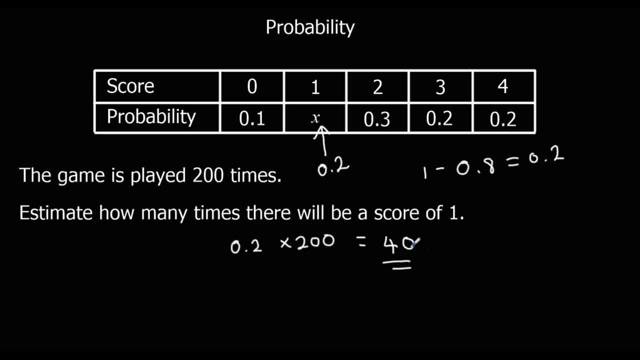 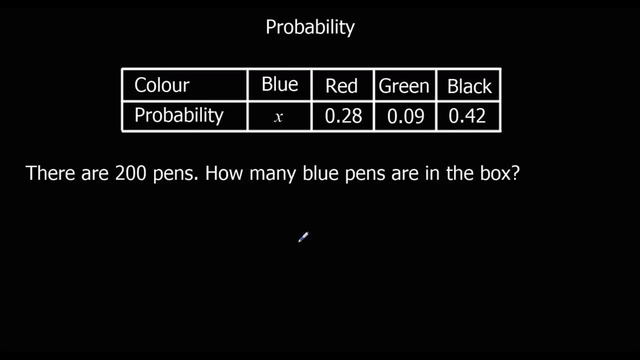 We divide it by 10 again, So it's 40. So we can estimate there'll be 40 ones scored. Okay, here's another example. So again we need to find the missing probability, So we need to add these ones up. 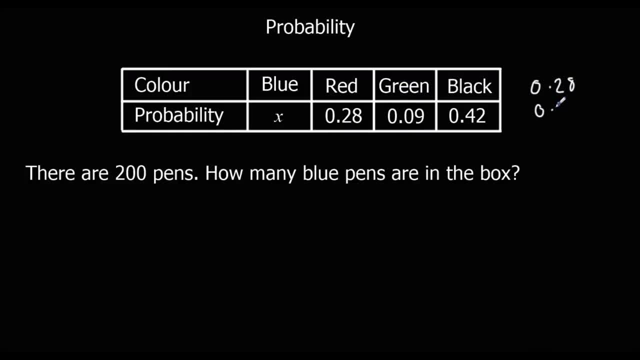 So we've got 0.28,, 0.09, and 0.42.. If we add them up Then we should be able to see what's missing. So 1 minus 0.79, that's 0.21.. 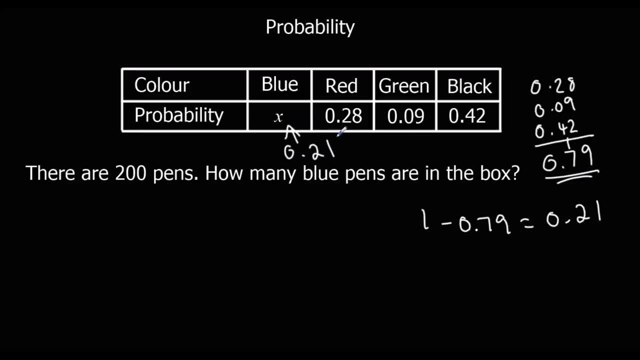 So the missing probability here is 0.21.. So there are 200 pens. How many are blue? So again 0.21 times 200.. So we can do 21 times 200. Which is 21.. So 21 times 2 is 42, with two 0s. 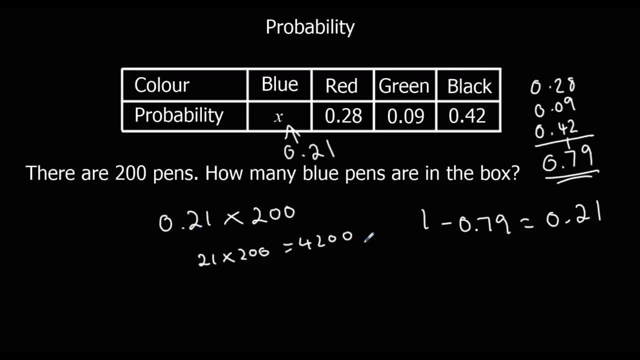 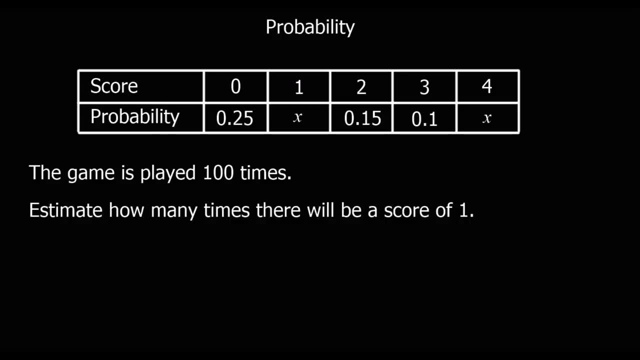 And there's two numbers after the decimal in the question, So two numbers after the answer, So it's 42.. Okay, pause the video, See if you can have a go at this one. Okay, so first we're going to find the missing probabilities again. 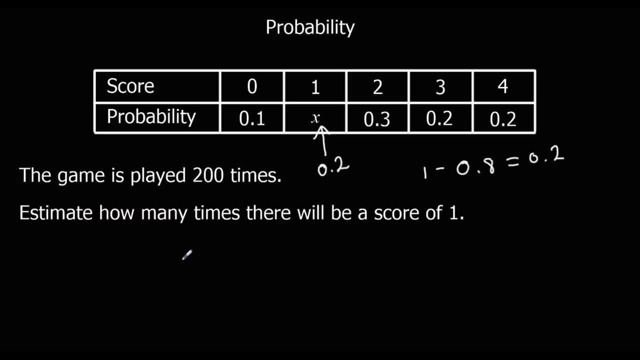 Now it says the game is played 200 times. Estimate how many times there will be a score. So it's this decimal, this chance, times 200.. So it's 0.2 times 200.. We want this fraction. If it was a fraction, it would be one-fifth, one-fifth of 200.. 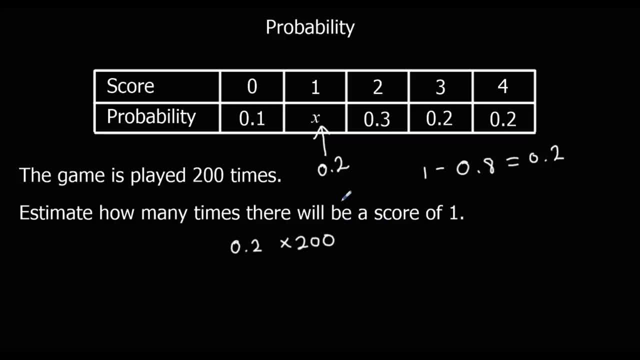 If it was a percentage: 20%, 20% of 200. So it's just 0.2 times 200.. So 2 times 200, that's 400.. But because it's 0.2, we take off a zero. 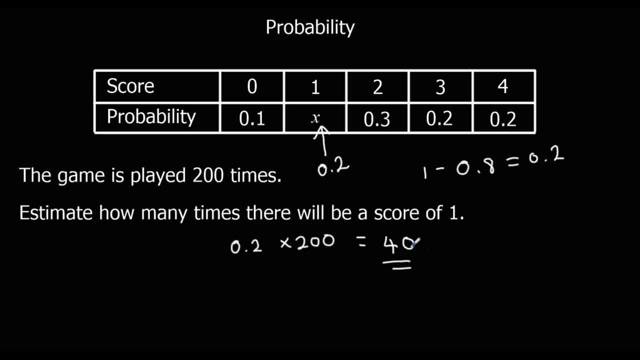 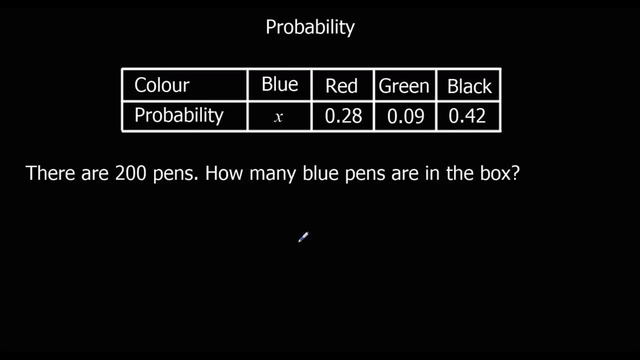 We divide it by 10 again, So it's 40. So we can estimate there'll be 40 ones scored. Okay, here's another example. So again we need to find the missing probability, So we need to add these ones up. 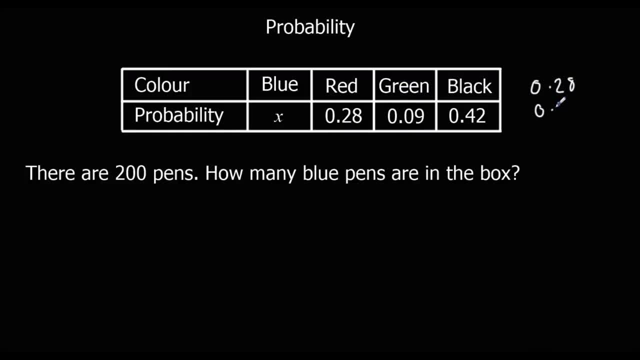 So we've got 0.28,, 0.09, and 0.42.. If we add them up Then we should be able to see what's missing. So 1 minus 0.79, that's 0.21.. 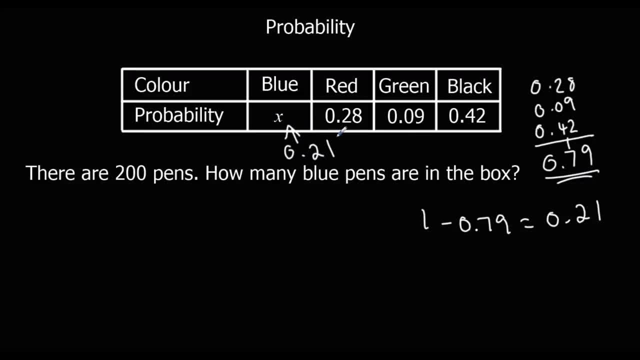 So the missing probability here is 0.21.. So there are 200 pens. How many are blue? So again 0.21 times 200.. So we can do 21 times 200. Which is 21.. So 21 times 2 is 42, with two 0s. 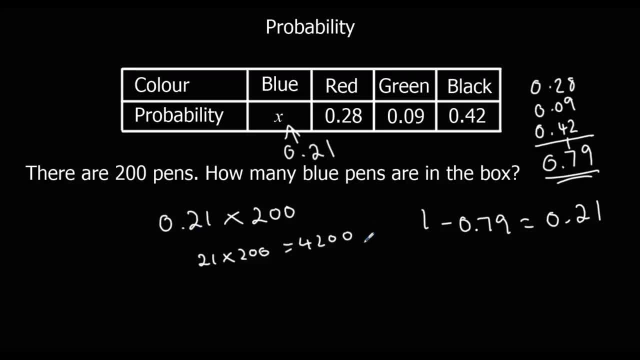 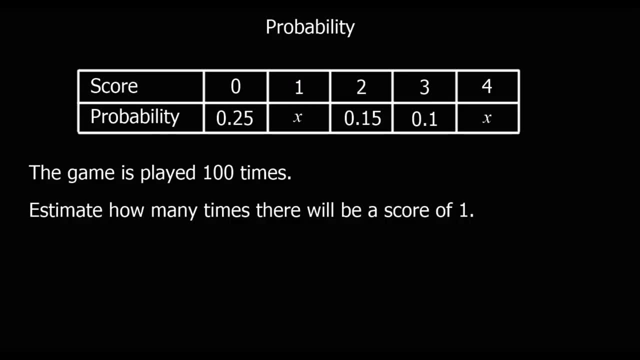 And there's two numbers after the decimal in the question, So two numbers after the answer, So it's 42.. Okay, pause the video, See if you can have a go at this one. Okay, so first we're going to find the missing probabilities again. 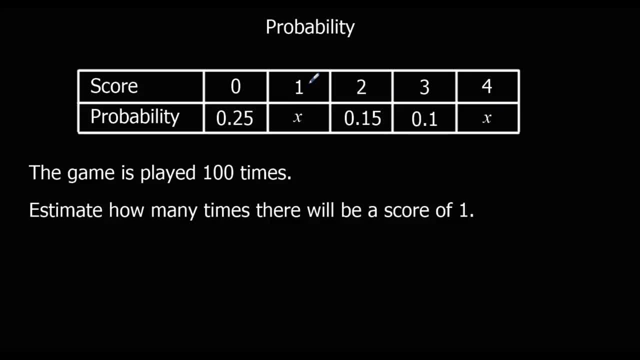 This time there's two Xs. That means they're the same. So the probability of 1 happening and the probability of 4 happening are the same. So we're going to add up what we've got so far. So this is 0.25 plus 0.15, is 0.4, plus 0.1, 0.5..